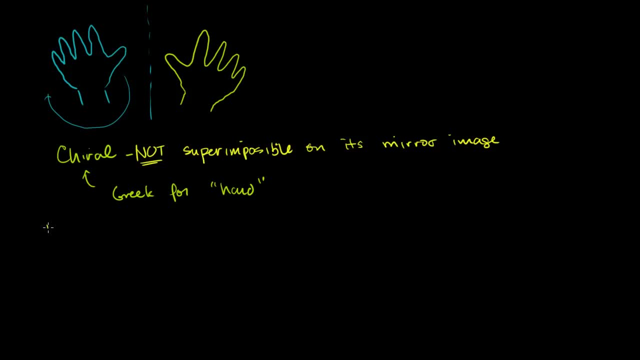 what we're talking about. there's two concepts here. There are chiral molecules and then there are chiral centers, or chiral- well, I'll call them chiral atoms. They tend to be carbon atoms, so sometimes they call them. 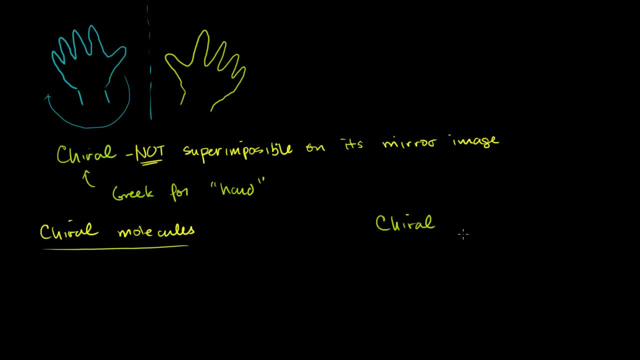 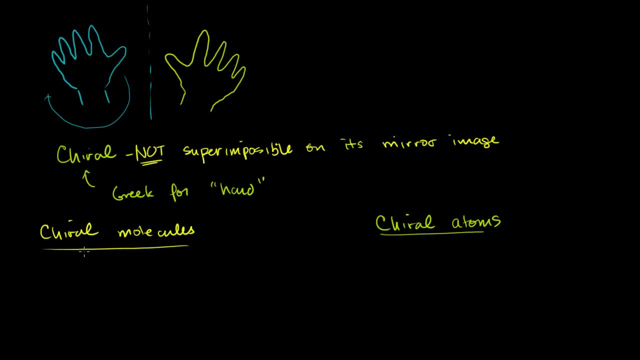 And then you have chiral atoms. Now, chiral molecules are literally molecules that are not superimposable on their mirror image. So, not, I'm not going to write the whole thing- Not superimposable, I'll just write the whole thing. 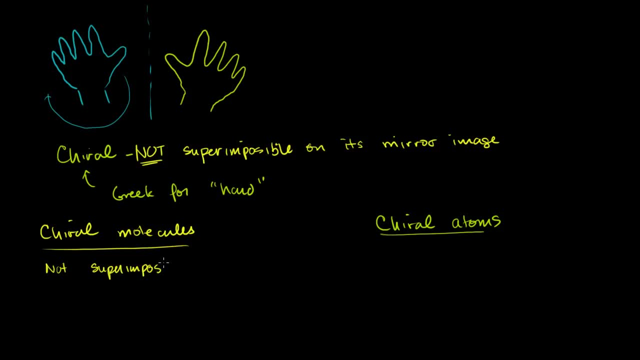 Not superimposable on mirror image. Now for chiral atoms. this is essentially true, But when you look for chiral atoms within a molecule, the best way to kind of spot them is to recognize that these generally- or maybe I should say usually- are carbons. 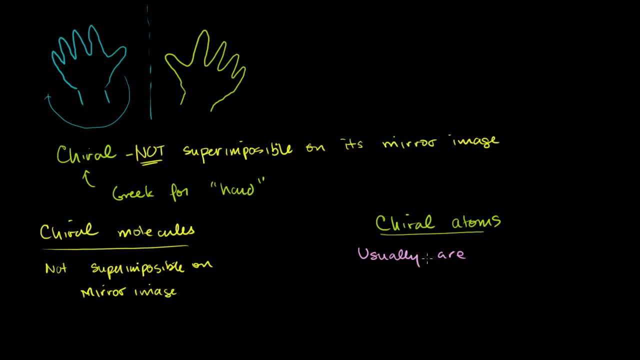 especially when we're dealing with organic chemistry. but they could be phosphoresces or sulfurs, but usually are carbons. are carbons bonded to four different groups, four different groups, different groups, And I want to emphasize groups, not just four different atoms. 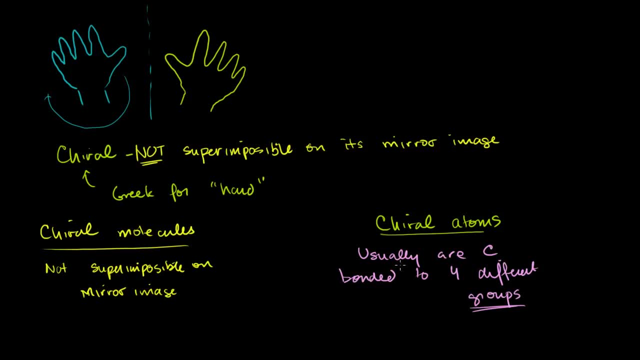 And to kind of highlight a molecule that contains a chiral atom or a chiral carbon. we can just think of one. So let's say that I have a carbon right here And I'm going to set this up, so this is actually a chiral atom. 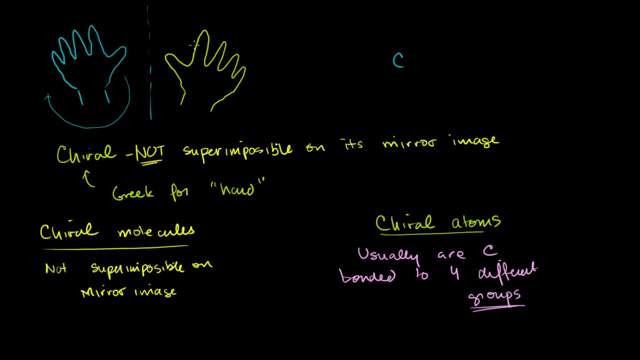 that the carbon specific is a chiral atom, But it's part of a chiral molecule, And then we'll see examples that are one or both of these are true. So let's say it's bonded. Let's say it's bonded. 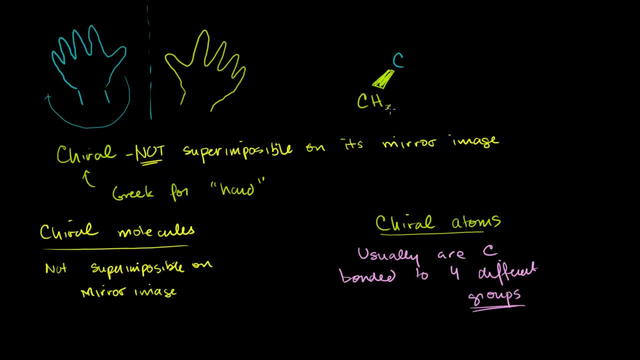 Let's say it's bonded to a methyl group. From that bond it kind of pops out of the page. Let's say there's a bromine over here. Let's say behind it there is a hydrogen, And then above it we have a fluorine. 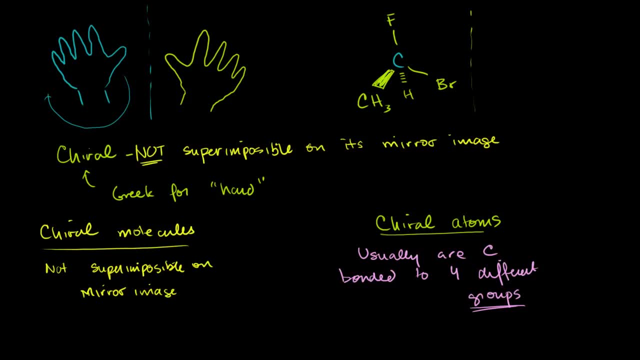 Now if I were to take the mirror image of this thing right here, we have your carbon in the center. I want to do that same blue, You have the carbon in the center And then you have the fluorine above the carbon. Then you have your bromine now going in this direction. 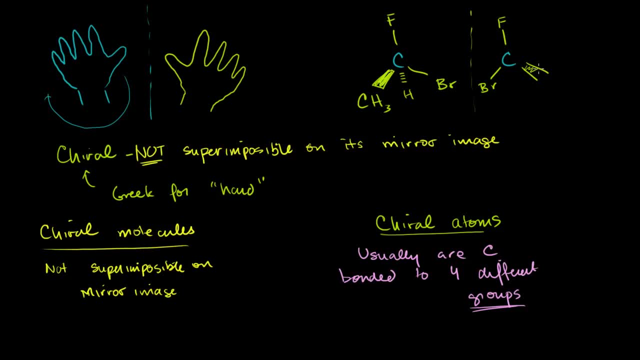 You have this methyl group. It's still popping out of the page, but it's now going to the right instead of to the left, so CH3.. And then you have the hydrogen still in the back. These are mirror images. if you view this as kind of the. 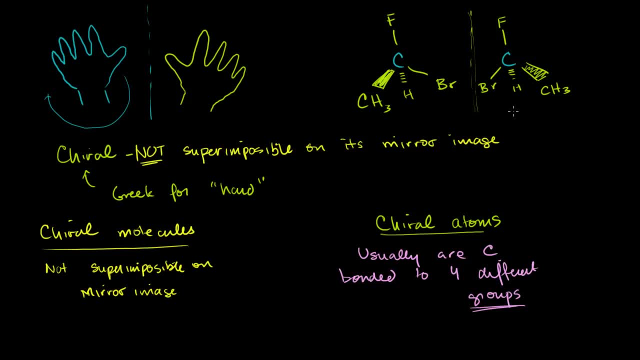 mirror and you can see on both sides of the mirror. Now, why is this chiral? Well, no matter how, and it's a little bit of a visualization challenge, but no matter how you try to rotate this thing right here, you will never make it. 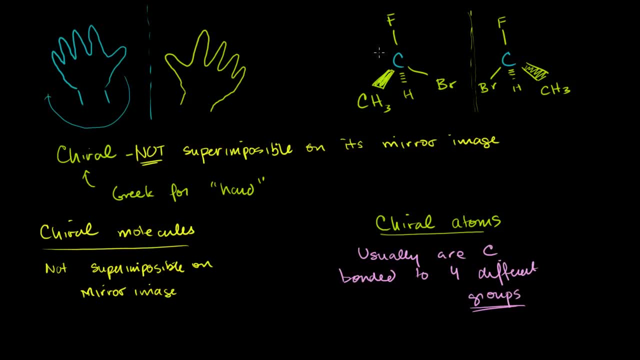 exactly like this thing. You might try to rotate it around like that and try to get the methyl group over here, to get it over there. So let's try to do that. But if we try to get the methyl group over there, what's going? 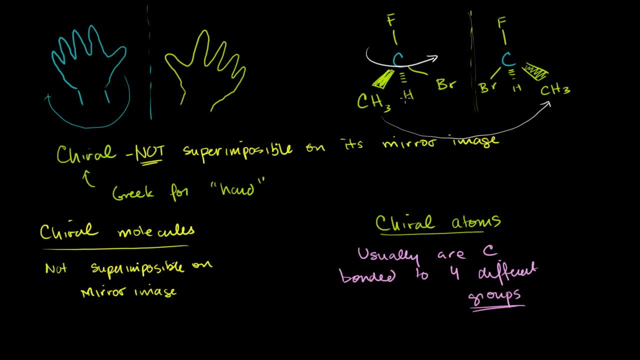 to happen to the other groups. Well then, the hydrogen group is going, or the hydrogen, I should say the hydrogen atom, is going to move there and the bromine is going to move there. So this would be superimposable if this was a 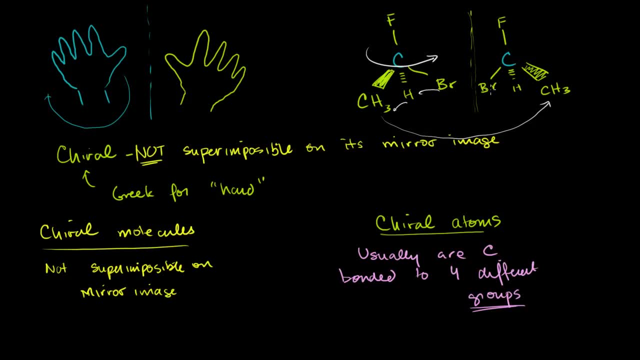 hydrogen and this was a bromine, but it's not. You can imagine that hydrogen and bromine are switched and you could flip it and do whatever else you want or try to rotate it in any direction, but you're not going to be. 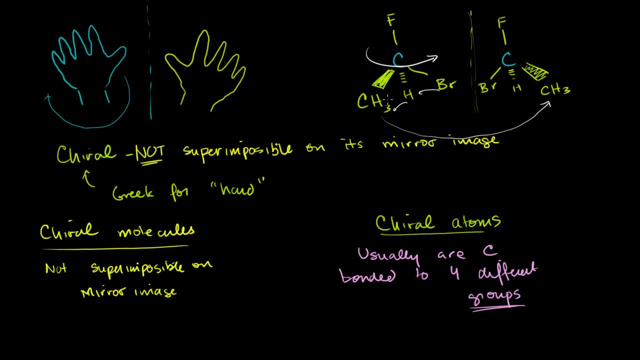 able to superimpose them. So this molecule right here is a chiral molecule and this carbon is a chiral center. So this carbon is a chiral carbon, sometimes called an asymmetric carbon or a chiral center. Sometimes you'll hear something. 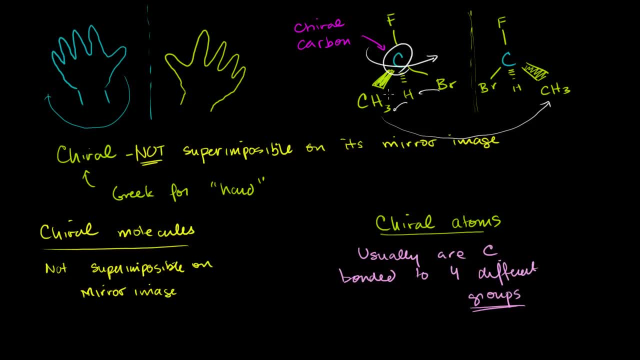 It's called a stereocenter. A stereocenter is a more general term for any point in a molecule that is asymmetric relative to the different groups that it is joined to. But all of these- especially when you're kind of in an introductory organic chemistry class, tends to be a carbon. 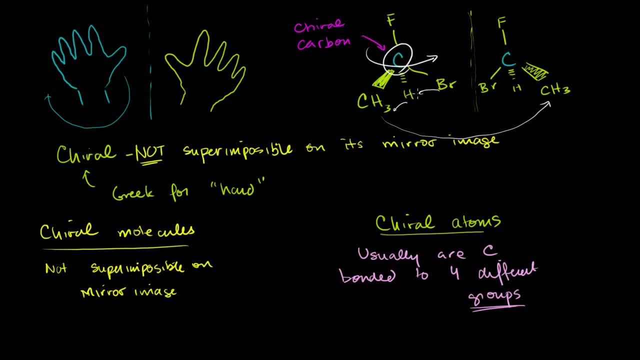 bonded to four different groups, And I want to stress that it's not four different atoms. You could have had a methyl group here and a propyl group here, and the carbon would still be bonded directly to a carbon in either case, But that would still be a chiral carbon and this would